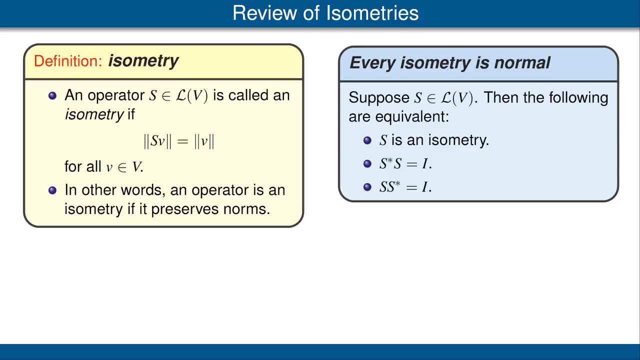 Then the following 3 conditions are equivalent. 1st condition s is an isometry. 2nd condition s: star s equals the identity operator. 3rd condition s: times s star equals the identity operator. Let's consider a consequence of this result. 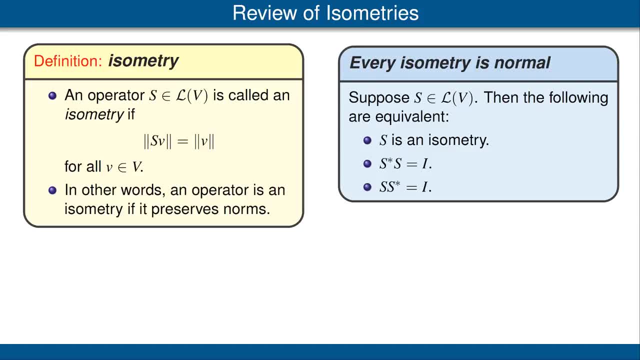 Suppose s is an isometry. here we see that s star s is equal to s s star, because both are equal to the identity operator. Thus s commutes with this adjoint, which means that s is normal. In summary, we have shown that every isometry is a normal operator. 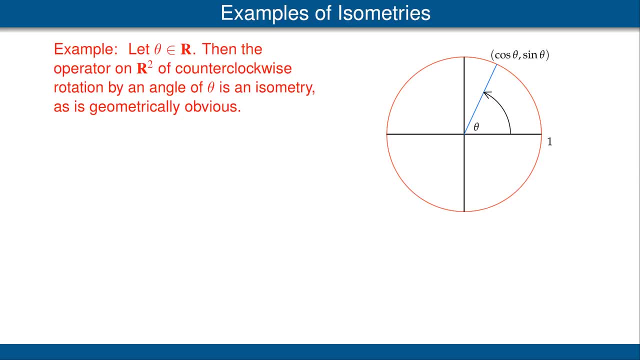 Let's look at a family of examples of isometries on R2.. Fix a real number, theta. Then the operator on R2 of counterclockwise rotation by theta is an isometry. That's geometrically obvious because rotation does not change the norm of a vector. 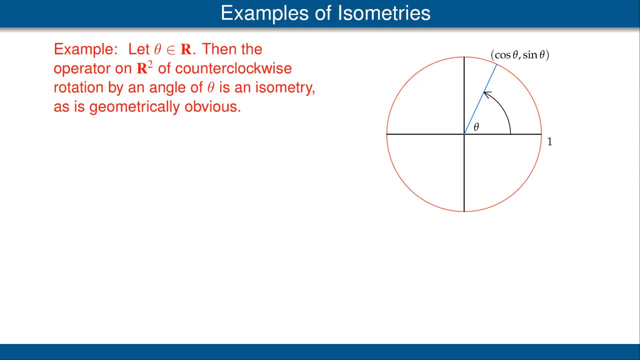 In the figure here, the one on the horizontal axis indicates that we are dealing with the unit circle in R2.. As you can see, if we rotate the point by an angle of theta counterclockwise, we get the point cosine, theta sine theta. In fact, this is the definition of the cosine and the sine. 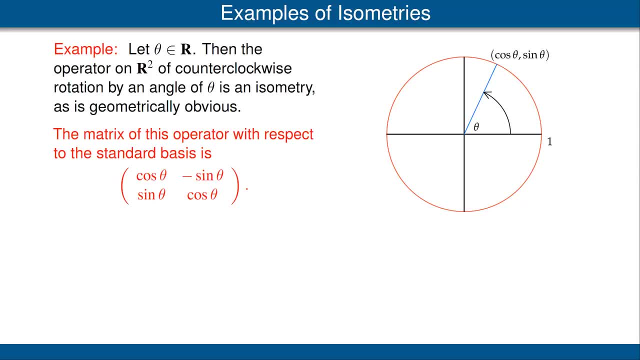 The matrix of this rotation operator with respect to the standard basis of R2 is shown here. The first standard basis vector is the vector and you can see in the first column the coordinates of the rotation cosine: theta, sine theta If theta equals zero. 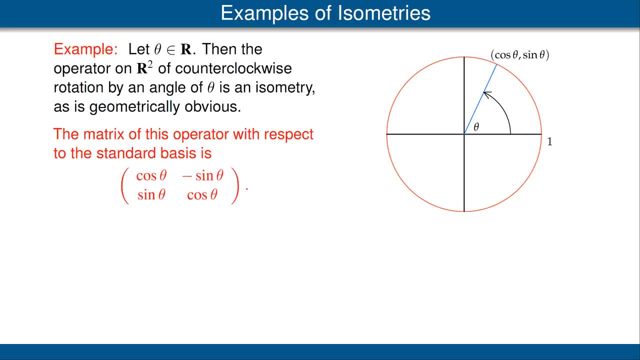 we just have the identity operator. If theta equals pi, then we have a rotation of pi radians or 180 degrees. That operator is the negative of the identity operator. However, if theta is not an integer multiple of pi, then clearly no non-zero vector of R2. 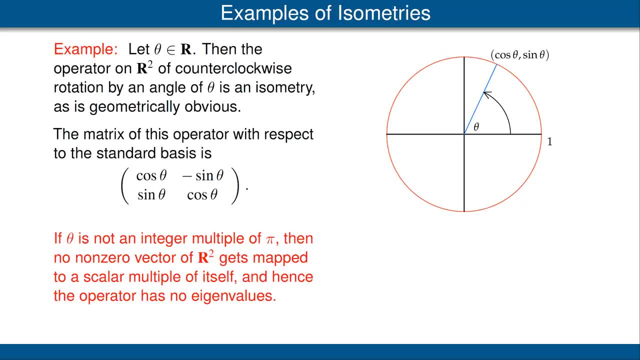 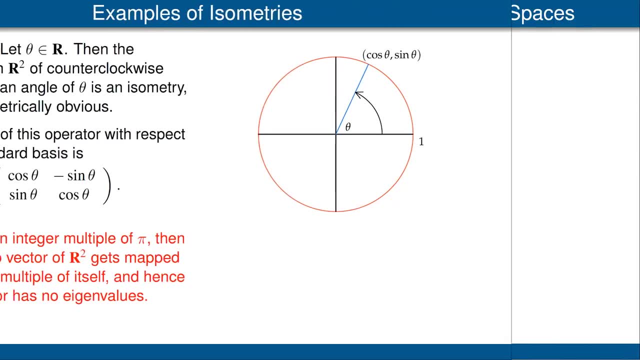 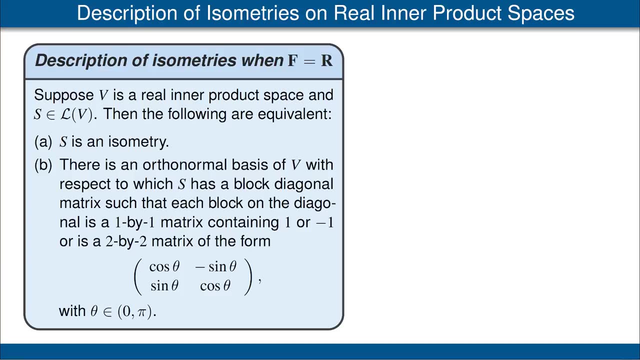 gets mapped to a scalar multiple of itself. Thus, if theta is not an integer multiple of pi, the operator has no eigenvalues. In a previous video we gave a complete description of isometries on a finite-dimensional, complex inner product space. 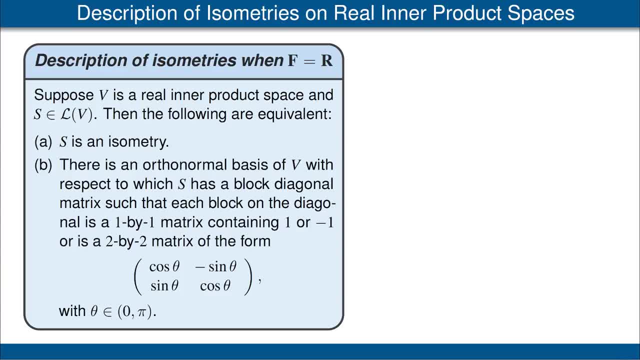 Recall that description. If we have an isometry on a complex inner product space, then there's an orthonormal basis of that complex inner product space, with respect to which the matrix of the isometry is a diagonal matrix and each entry on the diagonal. 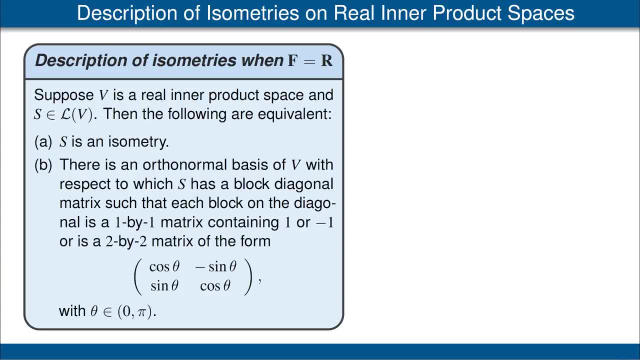 is a complex number with absolute value 1.. That description is not true on real inner product spaces. but now we can give a complete description of isometries on real inner product spaces. Here it is: Suppose V is a real inner product space and S is an operator on V. 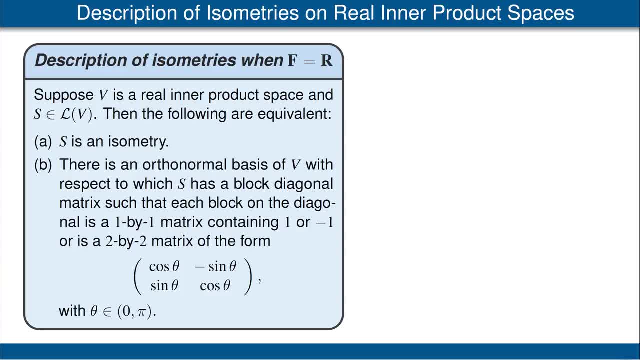 Then the following are equivalent: A- S is an isometry. Condition B is that there is an orthonormal basis of V, with respect to which S has a block-diagonal matrix such that each block on the diagonal is a 1x1 matrix containing either 1 or negative 1, or is a 2x2 matrix of the form shown here. 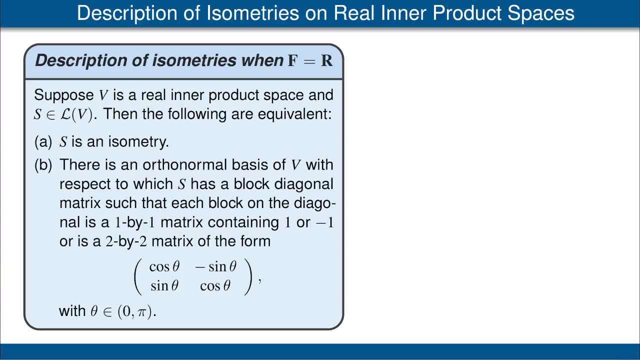 where theta is an angle in the interval from 0 to pi. If you think about Condition B, it says that an isometry on a real inner product space gives the decomposition of the vector space as a direction. This is a direct sum of subspaces and on each of those subspaces, 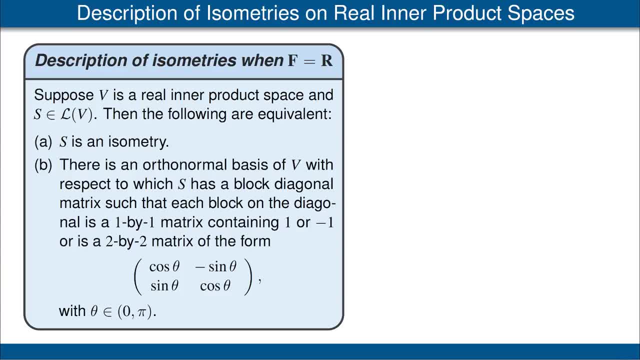 the isometry is either multiplication by 1, in other words, is just the identity, or is the negative of the identity, or is a rotation by some angle. Let's look at the proof that A implies B. Let's suppose that A holds, meaning that S is an isometry. 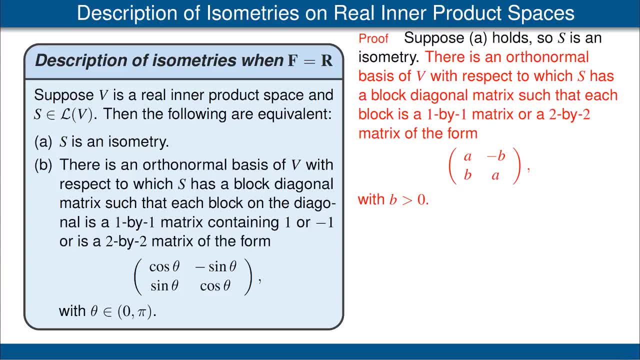 In particular, S is a normal operator and from a result in the previous video we can conclude that there is an orthonormal basis of V, with respect to which S has a block-diagonal matrix such that each block is a 1x1 matrix or a 2x2 matrix of the form shown here. 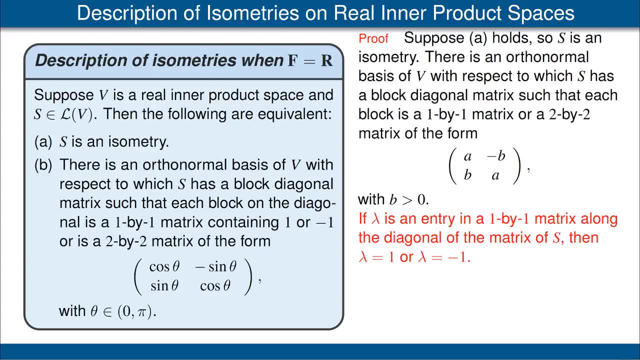 Let's think about this block-diagonal matrix description of S. If we look at a block that happens to be a 1x1 matrix, then because S is an isometry, the entry in that block has to have absolute value 1..